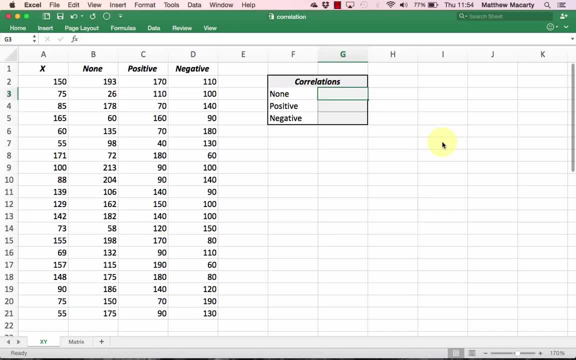 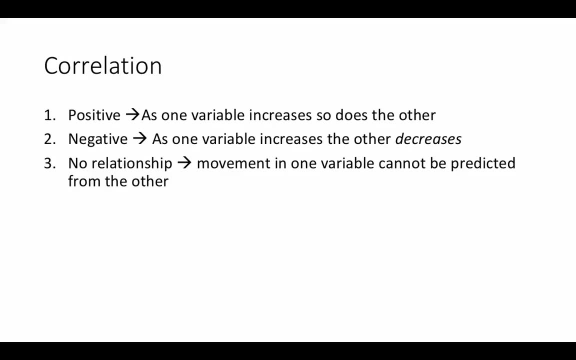 This kind of correlation is also known as Pearson's correlation or the Pearson product moment correlation. Correlation can be classified three different ways. There can be a positive relationship. This means as one variable increases, the other has a tendency to increase. There would be a negative relationship where as one variable increases, the other has a. 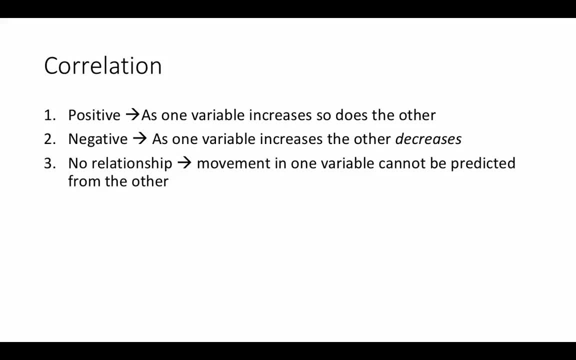 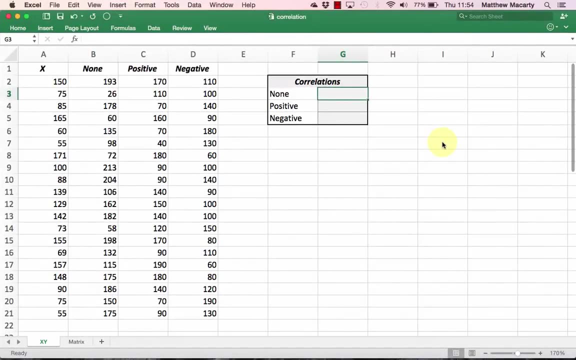 tendency to decrease. There may be no relationship at all, so movement in one variable couldn't be used to predict movement in the other. The correlation statistic is fairly tedious to calculate by hand, even with a calculator, But luckily Excel has a couple of ways to help us with this. 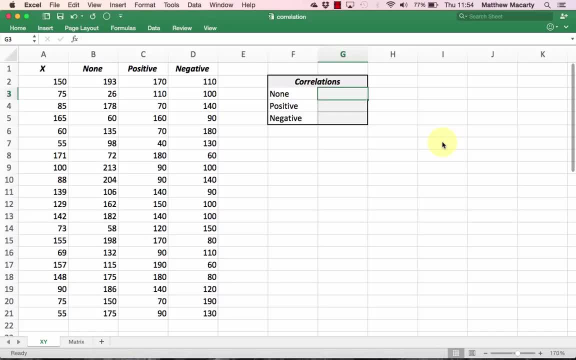 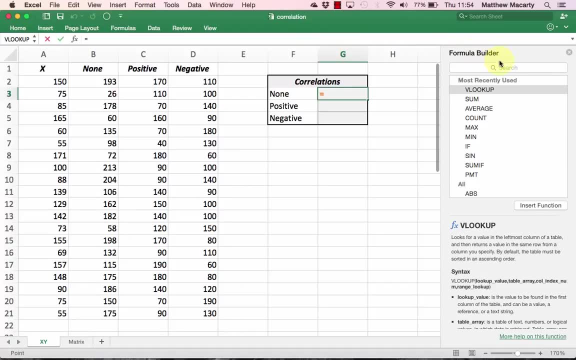 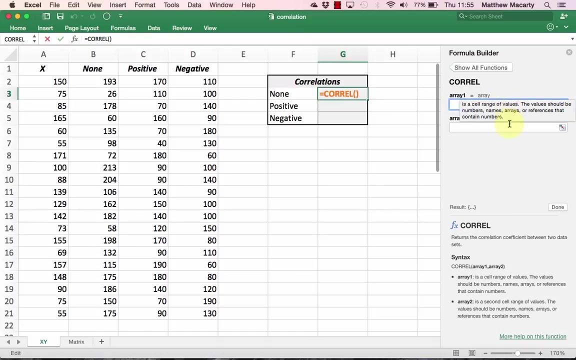 I'm going to show you how to use the Correl function. To get started, I'm going to click the fx button up next to the formula bar And in the formula pane I'm going to start typing correlation. Once Correl pops up, I'm going to double click to select it. 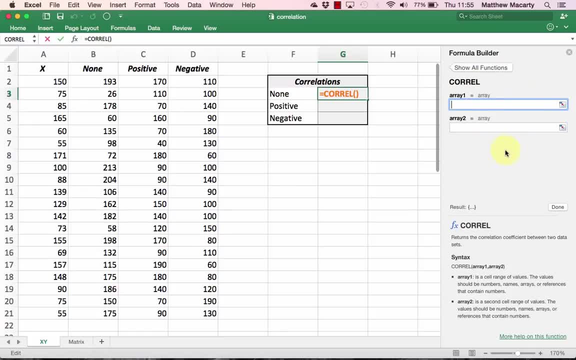 And the correlation will start The formula pane here. if you're using another version of Excel, it'll show the formula wizard. For array 1, I'm going to select the data in column A, labeled x. And. for array 2, I'm going to select the data in column B, labeled none. 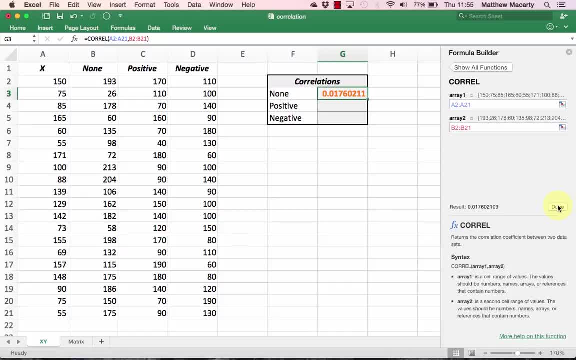 With that done, we can just click done, And we can see that these two variables have a correlation of very close to zero, 0.01.. And so we can safely conclude that, as the label predicted in column B, there is no correlation. 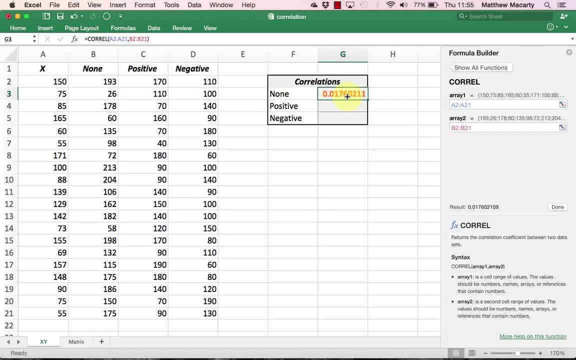 between the two variables. I'm going to repeat the process in G4.. So the formula pane should still be open. I'm just going to double click on Correl. I'll select the data in column A again, And for array 2, I'll select the data in column C.